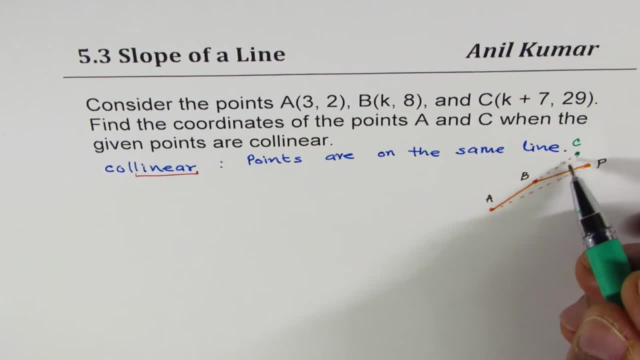 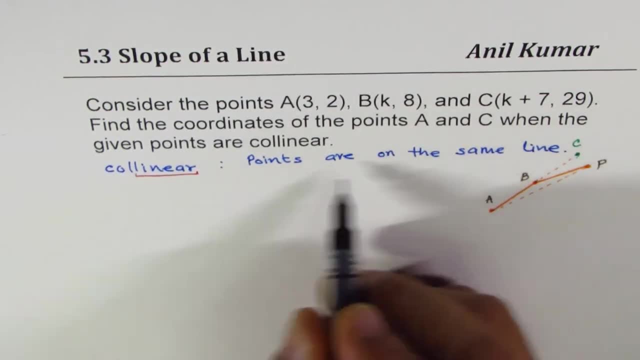 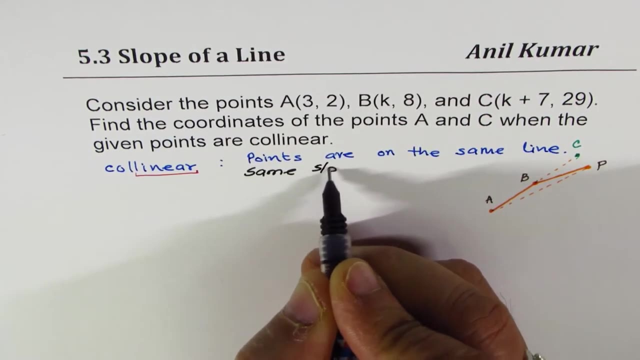 So you can check slope between any two points to ensure that they are collinear. So the concept here is points will share same slopes, So we are looking for same line means same slope, So that helps you to find the points correct. 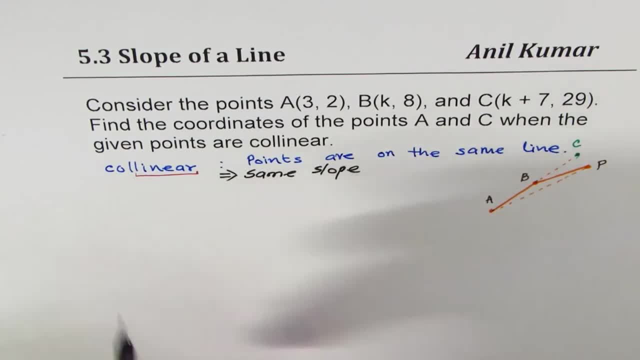 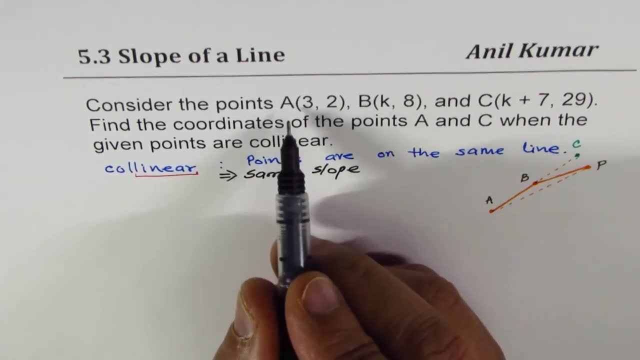 So let's find slope between two points. So we should definitely cover a point which is totally given to us. A is 3, 2.. So we'll find, in this case, slope from A to other two points. 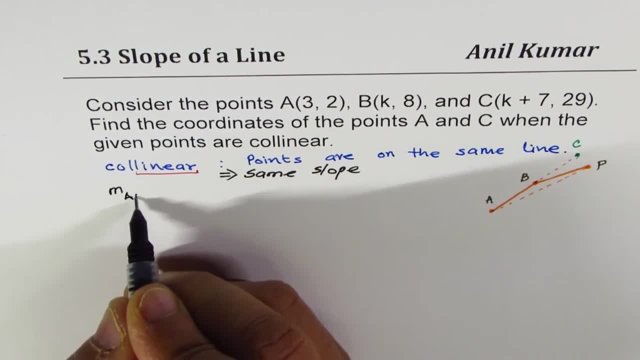 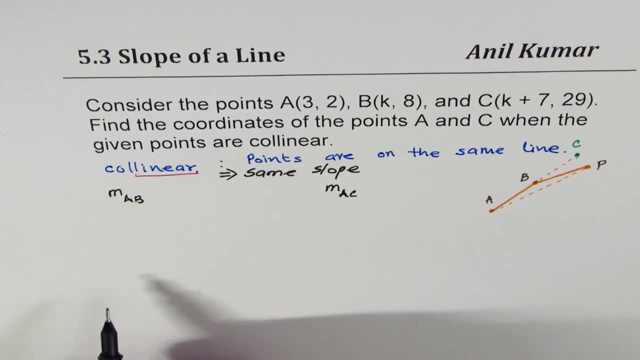 So basically, we'll try to find the slope between A and B, And we'll also find slope between A and C, And then we'll We'll equate them. That's the whole idea. So what is the slope between A and B? 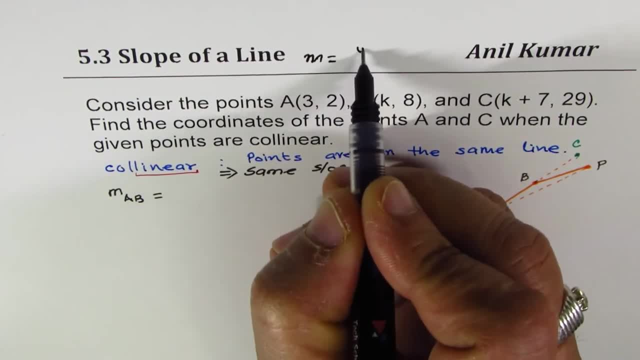 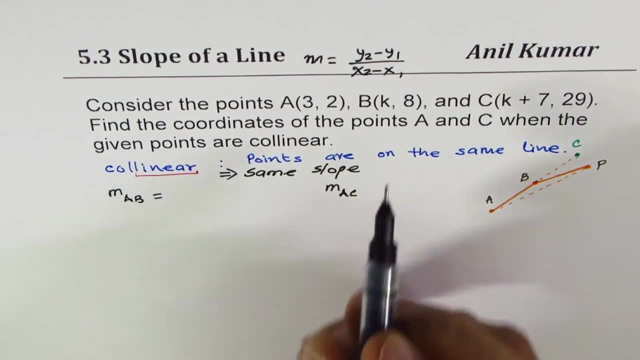 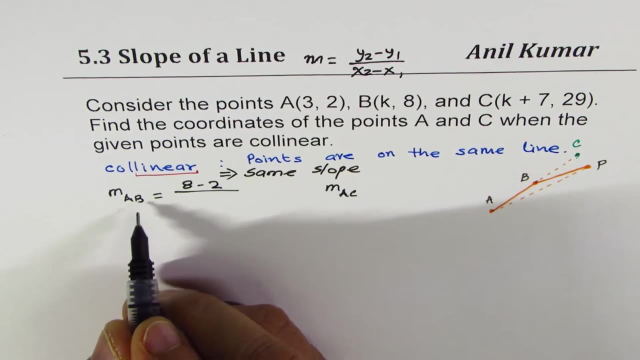 The formula for slope, as you know, is: M equals 2.. Change in Y divide by change in X, correct? We'll use this formula to find slope. So A and B: 8 minus 2.. When you write A and B, then A is the first point and B is the second point, right? 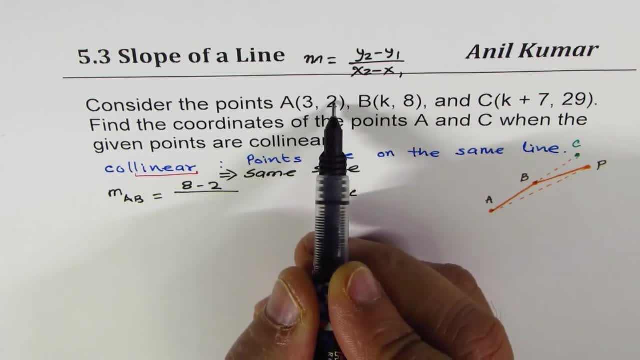 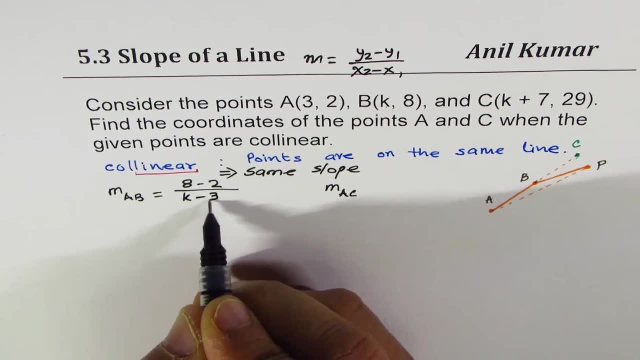 Okay, So A and B, 8 minus 2, Y2 minus Y1, divided by K minus 3, X2 minus X1.. Now that gives you 8 minus 2 is 6 over K minus 3.. 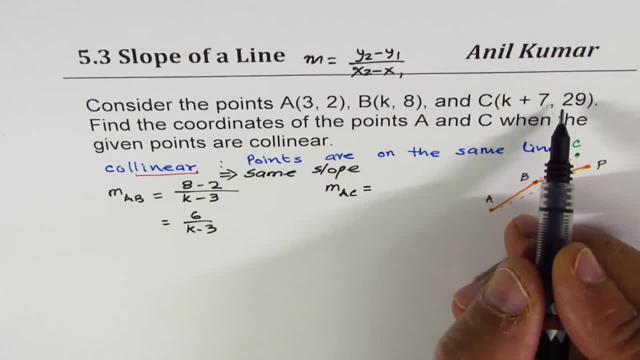 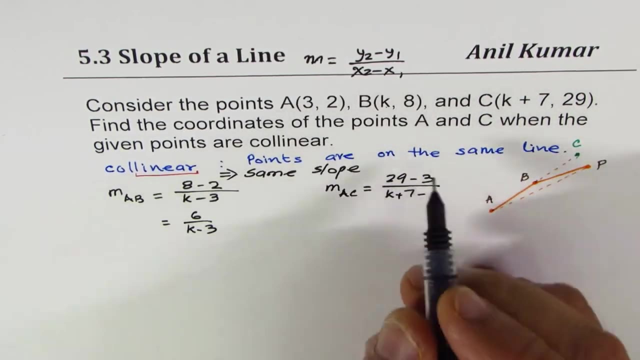 For AC A to C: 29 minus 3, divided by K plus 7.. So you have to write K plus 7 as such Minus. I'm sorry, 29 minus 2, sorry. K plus 7 minus 3, right. 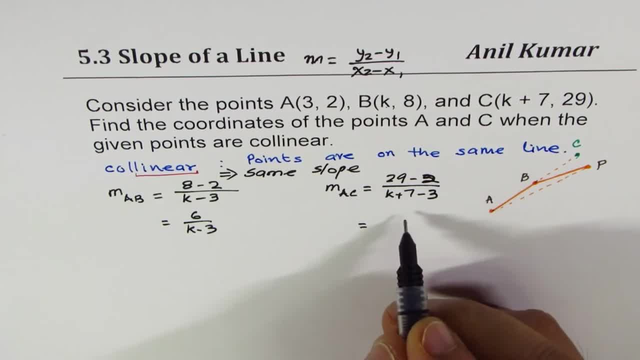 This is the Y2 value And that simplifies to 27 over K plus 4, right, So this is A to C Slope between A to B is 6 over K minus 3.. Now for them to be collinear. 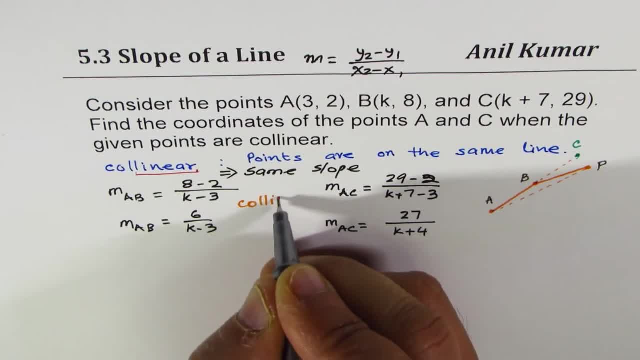 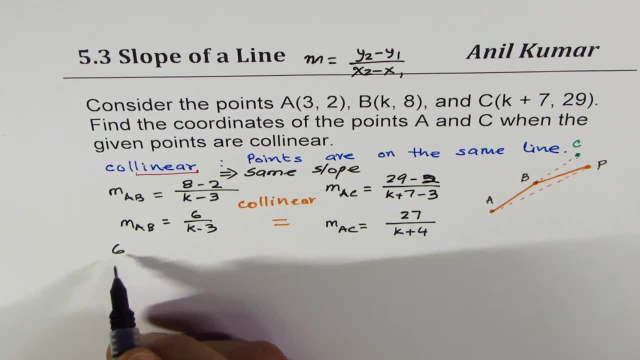 So when you say They are collinear, That means these two slopes are equal right? So we can form an equation which is 6 over K minus 3 equals to 27 over K plus 4.. Now you can actually simplify this a bit. 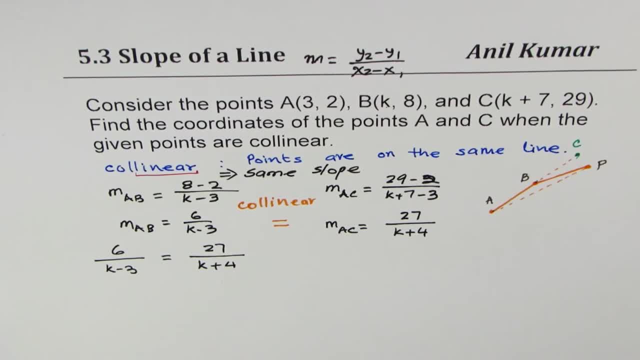 You can divide both by 3, less 2, right, It's easy. right, I mean it's better to simplify, Because when we just cross multiply, we are left with bigger numbers. So divide by 3,. we could write this as: 3 times 2 is 6, and 3 times 9 is 27.. 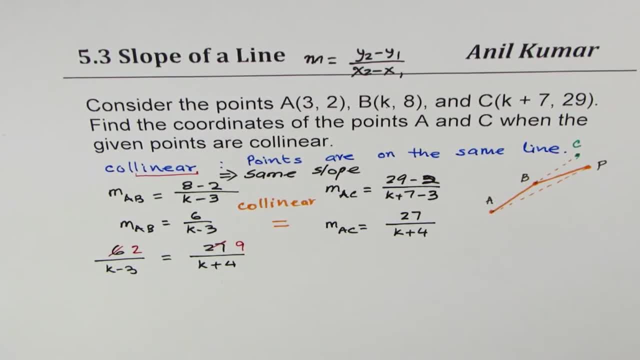 Is it okay? So first we'll simplify- It's a good practice to simplify and then do- And now we'll cross multiply. So we'll get 2 times K plus 4 equals to 9 times K minus 3.. 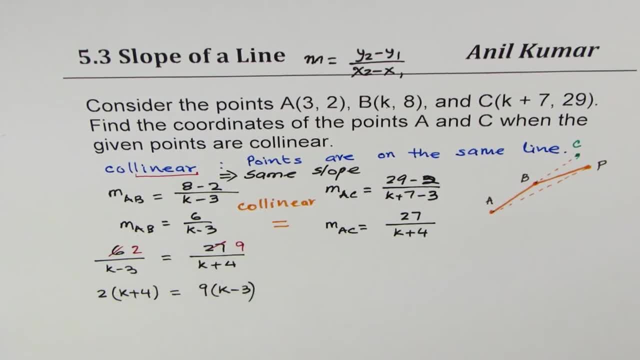 Even if you skip this Step, you'll get the same values. We are using calculators, so no problems. So we get 2K plus 8 equals to 9K minus 27.. So at this stage I've applied distributive property. 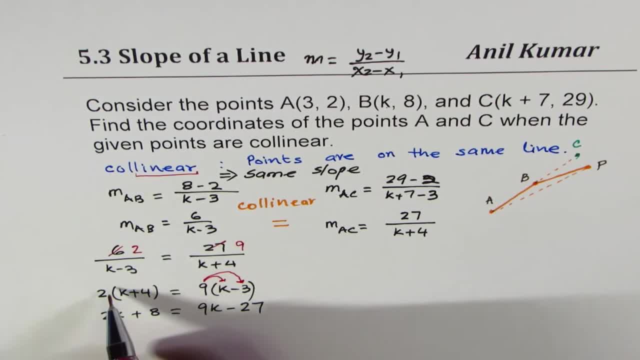 You have to multiply both the terms over the term outside. So that is the distributive property which you have learned. To solve for K we should bring Ks together and the constants together. So bringing 27 to the left makes 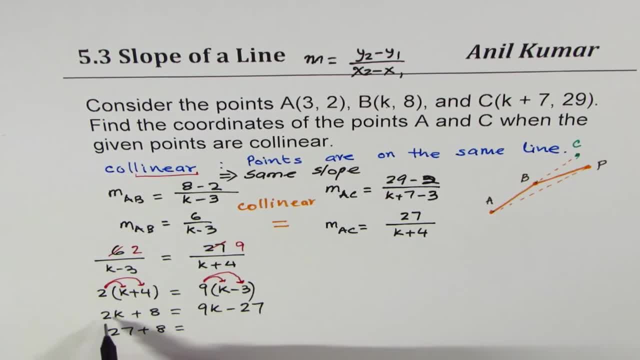 Let's say positive, 27 plus 8 equals to that will be 9K minus 2K, Is it okay? Let me take all this to the right side and to find the value of the K. So 9K minus 2K is 7K and 27 plus 8 is 35.. 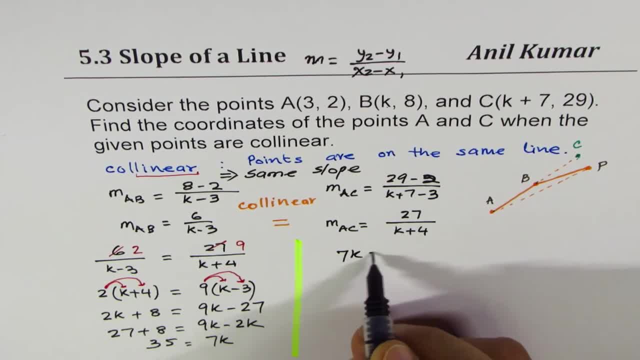 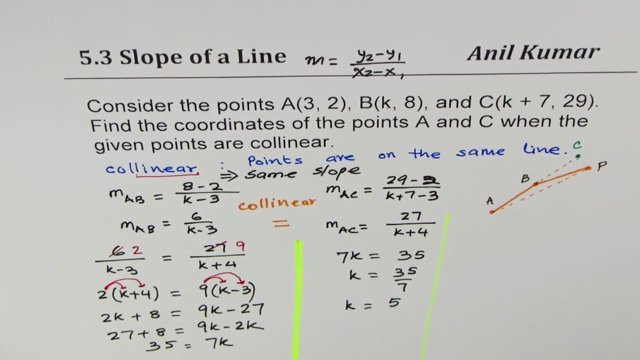 So we have 7K equals to 35, or K is equal to 35 divided by 7. So we get K as equals to 5.. Once you find the value of K, you can find both the points correct.